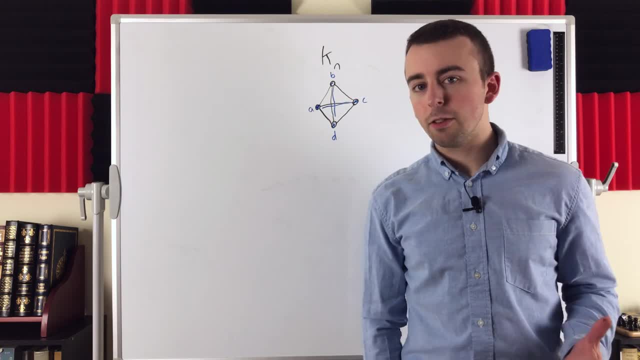 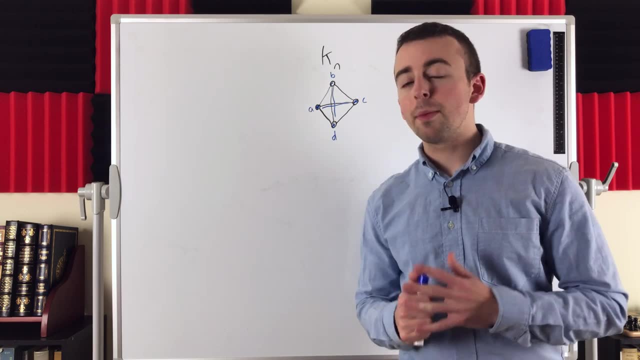 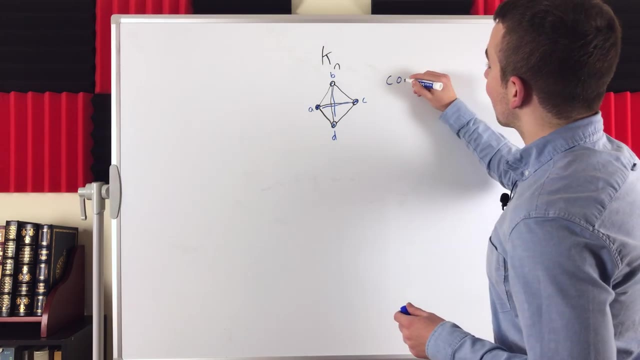 So we're trying to count the number of edges in a complete graph on n vertices, which is the same as counting the number of ways we can pick two vertices from a collection of n vertices, and perhaps that language makes you think about something, something called combinations. 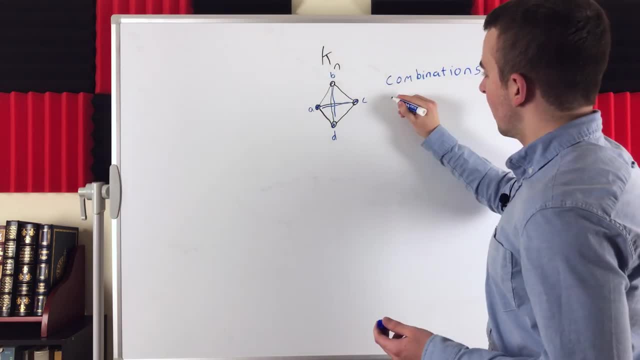 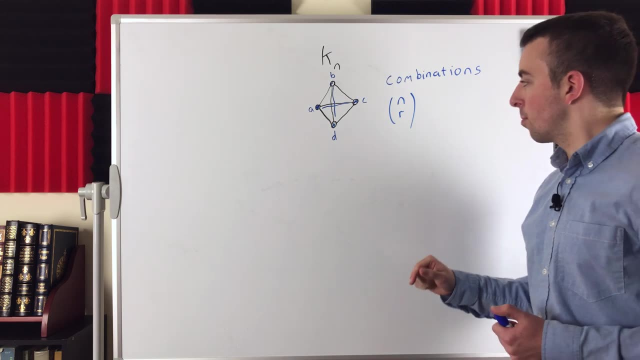 You might remember this if you've studied the language of combinations, If you've studied some combinatorics. this is called a binomial coefficient. It's the number of ways of selecting r objects from a collection of n objects. It's the number of combinations. 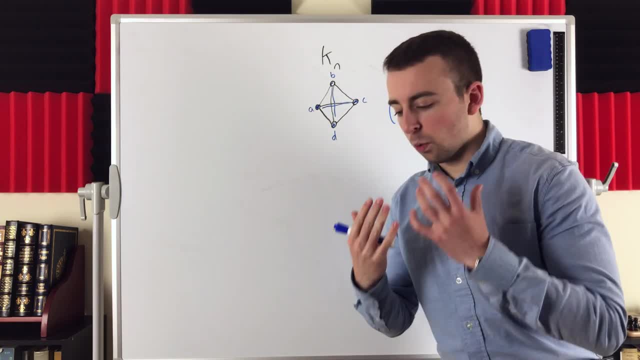 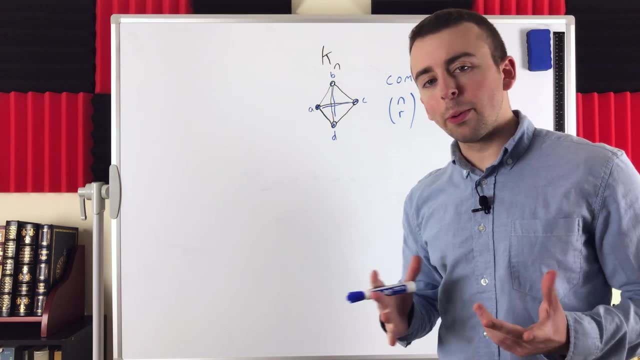 so the order doesn't matter. We're just sort of interested in what's in the combination, what's in the collection. We're not interested in order. Now, of course, if we were talking about directed graphs we'd be a bit more interested in order. but we're not. We're 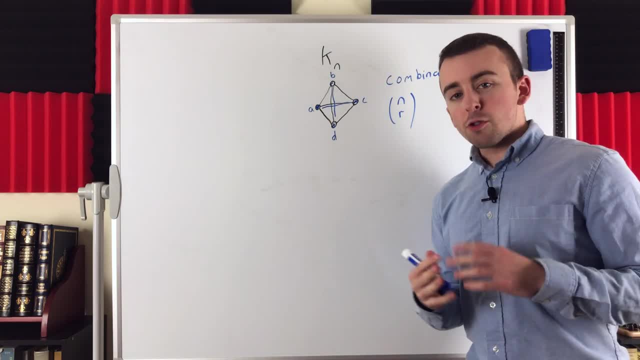 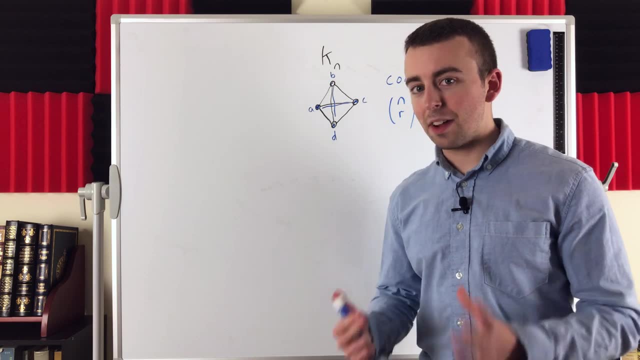 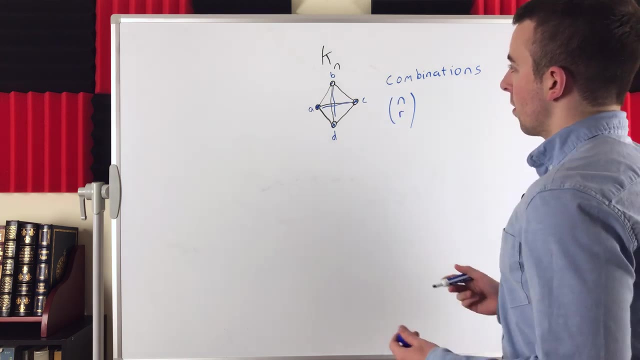 interested in simple, undirected graphs. So this is an equivalent problem: trying to count the number of ways we can select two vertices from a graph with n vertices. That's the number of edges it can have. So the solution falls out very naturally from that. If our graph has n vertices. 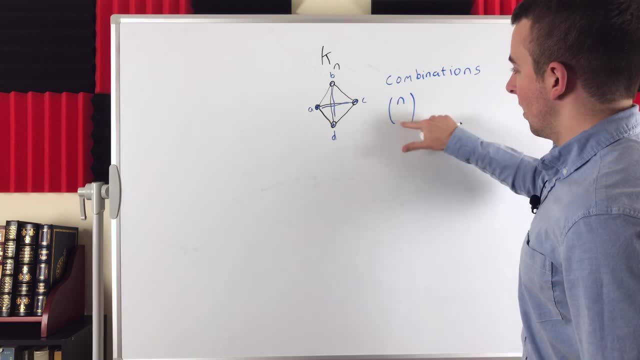 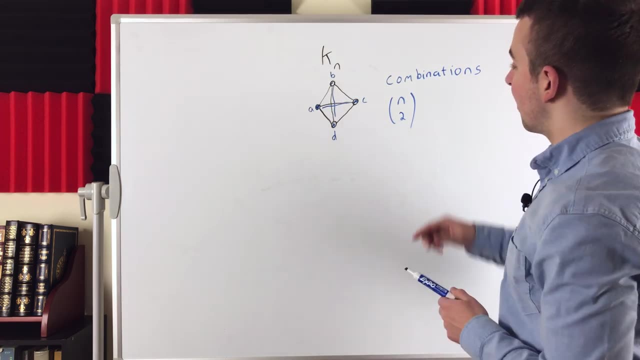 how many edges can it have? Well, it can have n choose 2 edges, and that's how that's read: n choose 2.. In this case, it's the number of ways we can select n vertices from a collection of n vertices. 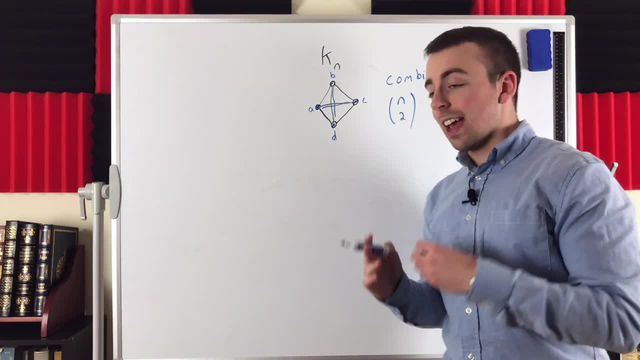 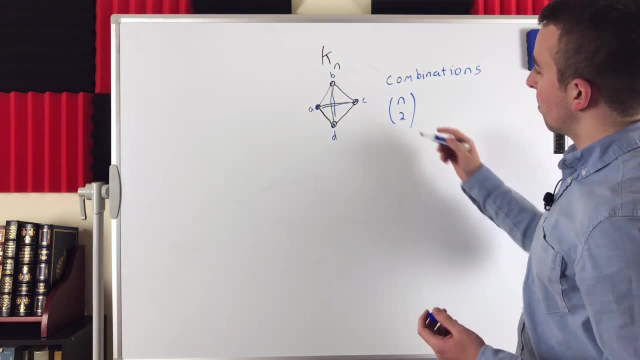 and that's how we can select two vertices from a collection of n vertices. Every pair of those vertices will make an edge, and that's the total number of edges we can have. That's the total number of edges in a complete graph with n vertices. Now, what is this actually equal to? 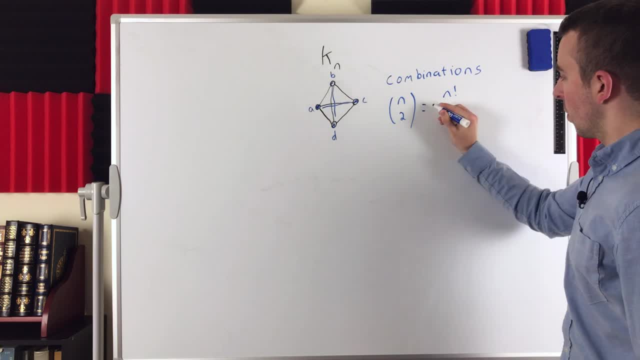 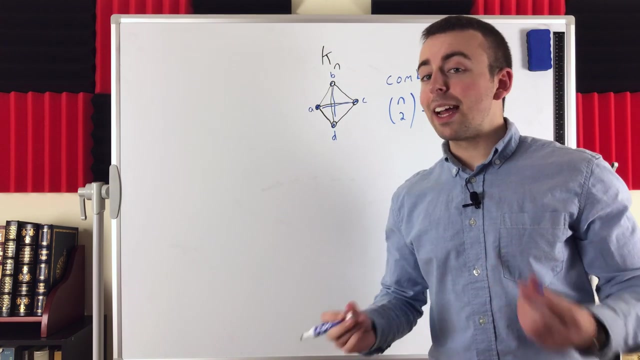 What's the formula? It's equal to n factorial divided by 2 factorial, multiplied by n minus 2 factorial. And if you're pretty familiar with combinations and why this formula works, then you're going to find that this formula can seem fairly beautiful and make a lot of sense to you. 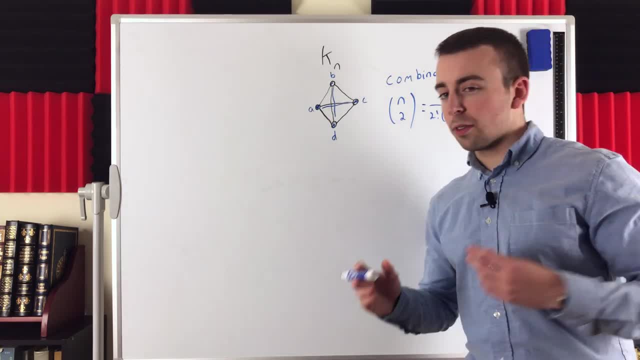 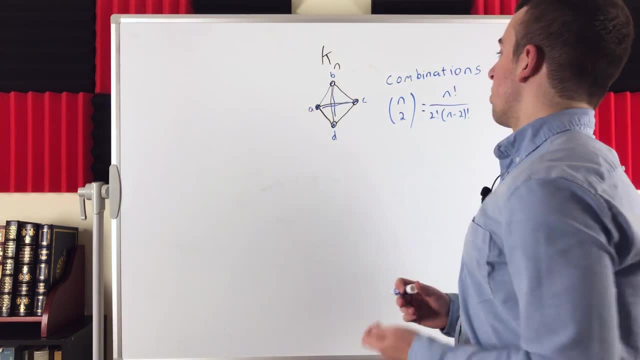 If you aren't as familiar with this, then of course you could go study it a little bit to get more familiar with it. but the next explanation we'll cover in the next lesson will perhaps be more interesting to you, because it's really just talking about graph theory and we don't have to. 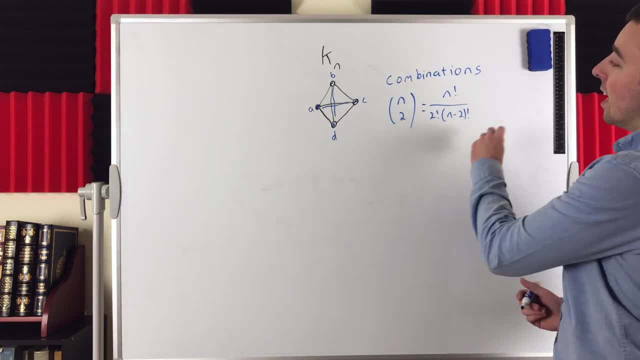 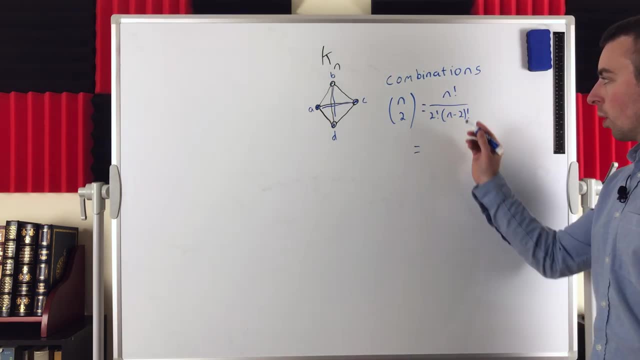 use combinations. But so this is the number, This is the number of edges in a complete graph with n vertices, and we can actually simplify it a little bit. So let's do that. What do we have in the numerator? We've got n factorial, which is n times n minus 1 times n minus 2, and so on all the way down to a. 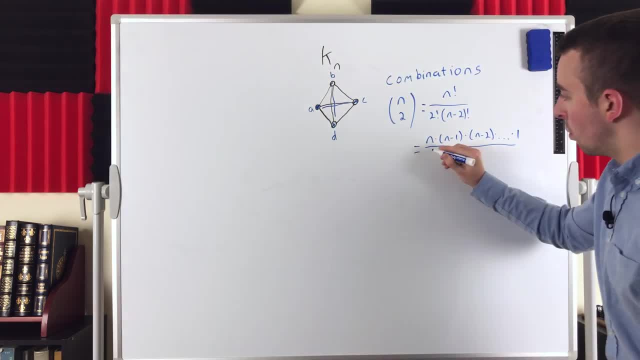 multiplication by 1.. And then in the denominator we've got 2 factorial, which is 2 times 1, which is just 2, multiplied by n minus 2 factorial, which is n minus 2, and so on down to a multiplication by: 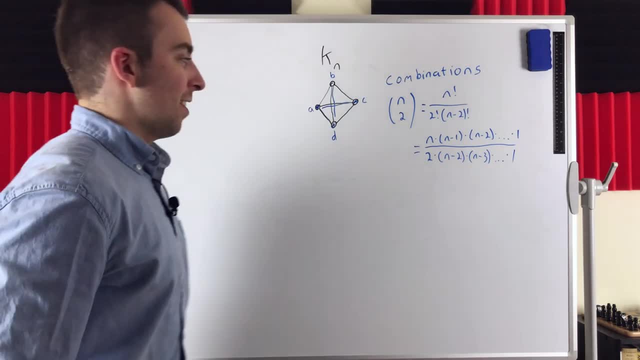 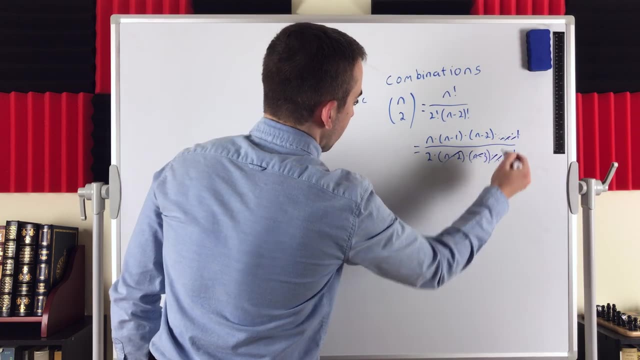 1. You can see it's going to be a whole lot of cancellation there. all right, Our n minus 2s cancel out. n minus 3s, all of those terms are going to cancel out. We're just left with. we're just left. 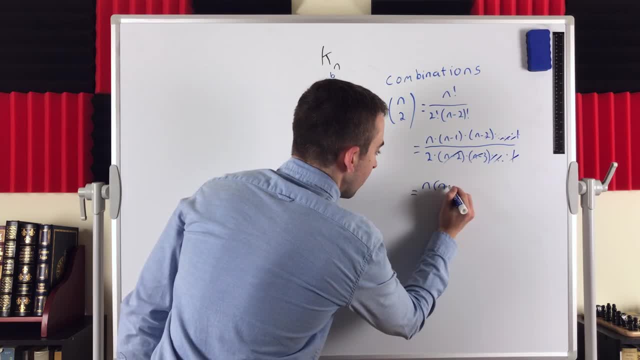 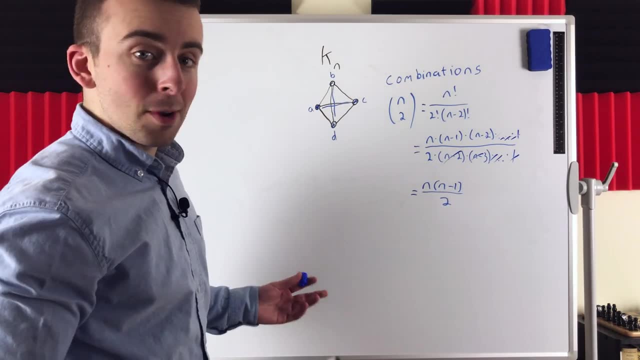 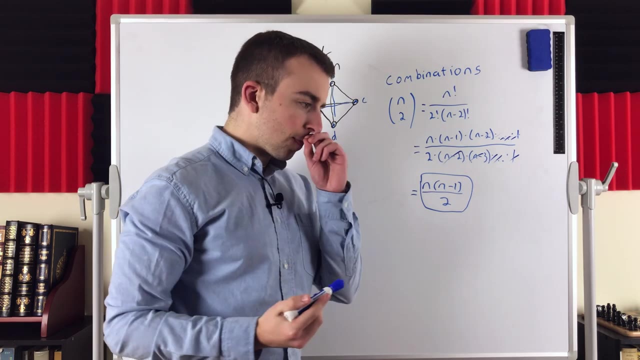 with n times n minus 1 in the numerator- trying to stay out of the way of the writing here- and then in the denominator, all we're left with is 2.. Pretty beautiful, So that's the number of edges in a complete graph with n vertices. Again, the reasoning is: it takes two vertices to make an. 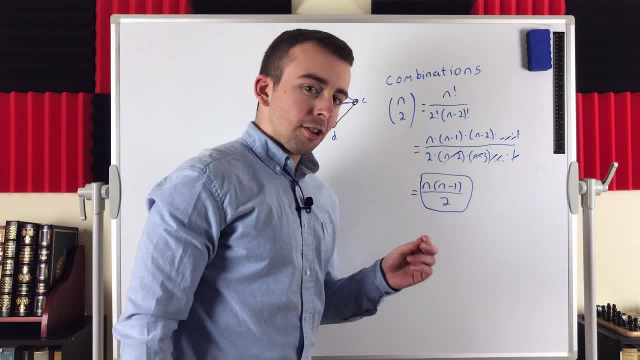 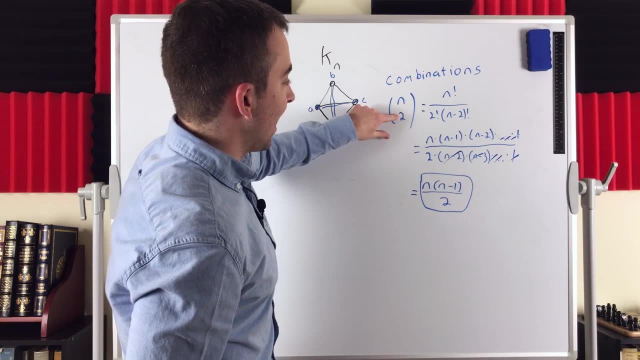 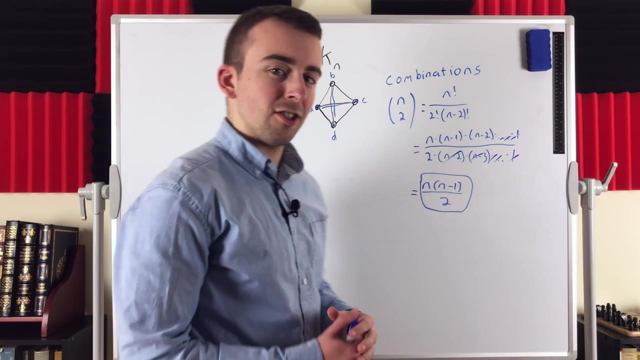 edge. Two vertices define an edge. So the total number of edges we can have in a graph with n vertices is the total number of ways we can select two vertices from a collection of n vertices, And that number, the total number of possible edges, is the number of edges that are in a complete graph, because a complete graph on n 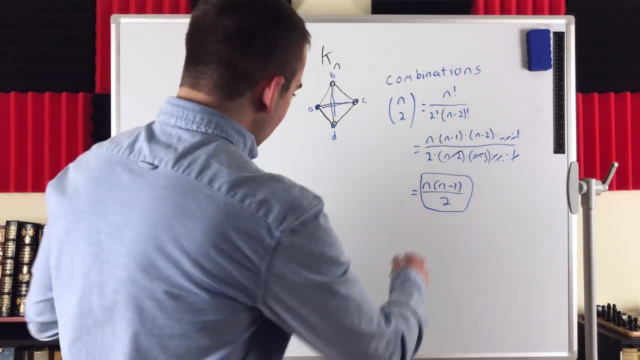 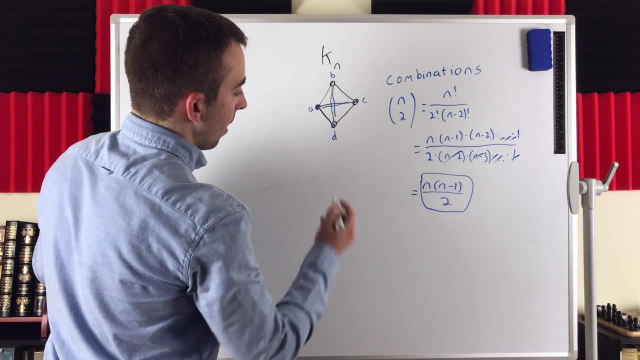 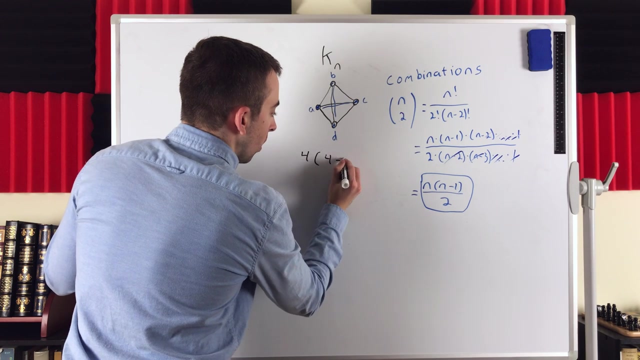 vertices has every possible edge. So let's quickly try applying this formula to our example with four vertices. Since this complete graph is a complete graph, we're going to have to apply this formula to our example. So if a complete graph has four vertices, it should have 4 multiplied by 4 minus 1 over two. 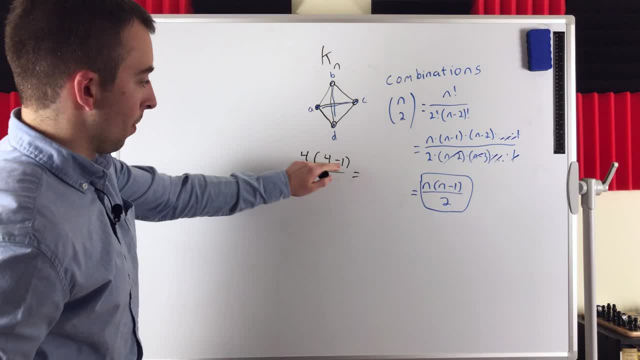 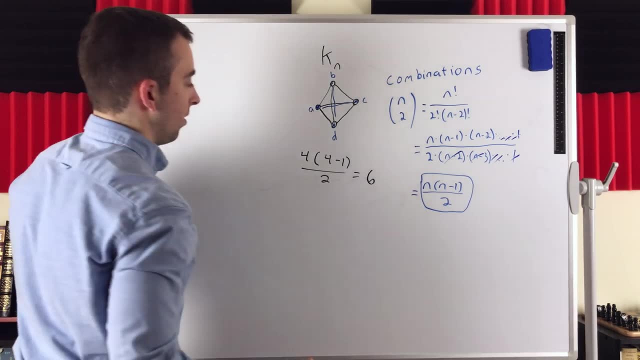 edges. And what's that? equal to? Well, 4 minus 1 is 3,, so that's 4 times 3, which is 12, divided by 2, which is 6.. Now, if we count those edges, just switch colors again to purple. how many edges do?